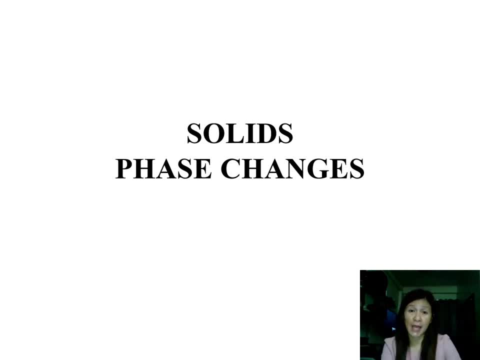 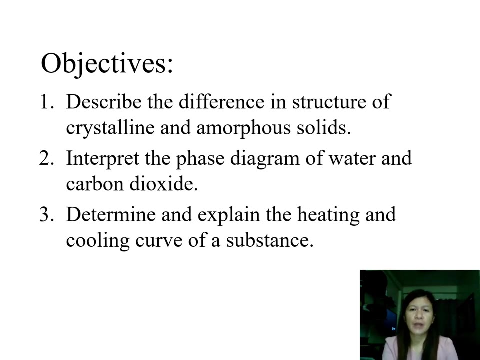 Hello class, welcome to our general chemistry 2 class. For this video we are going to discuss two subtopics: One is solids and the other is phase changes. For the objectives we will have: describe the difference in structure of crystalline and amorphous solids. to interpret the phase diagram of water and carbon dioxide. and three, determine and explain the heating and cooling curve of a substance. 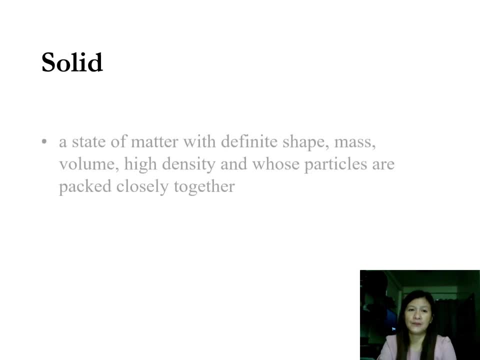 Let's first define a solid. What is a solid? A solid is a state of matter with definite shape, mass, volume, high density and whose particles are packed closely together. So we have emphasized in the last videos that solids are different from liquids and gases in such that particles in solids are closely packed together. 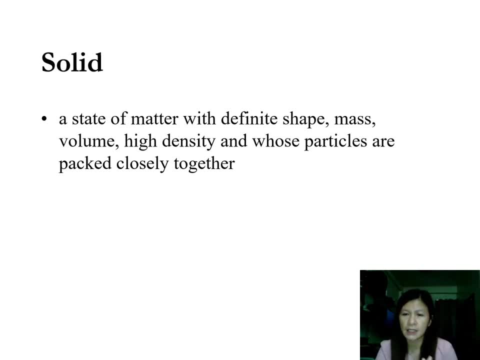 That's also the definition. That's also the reason why it has high density, because of the greater number of particles occupying a given space. So these are the common characteristics or properties of solids. when compared to liquids and gases, Solids may be categorized into two. 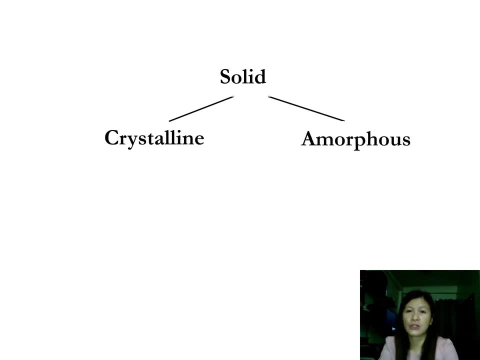 They may be crystalline solids or amorphous or non-crystalline solids. Crystalline solids are those that possess rigid and long rigidity. They are those that are in range order and whose particles occupy specific positions. Non-crystalline solids or amorphous solids are those that lack well-defined arrangement and long range order. 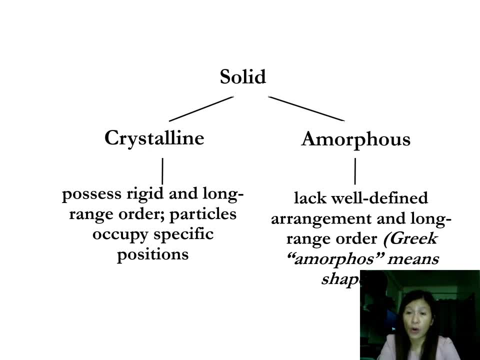 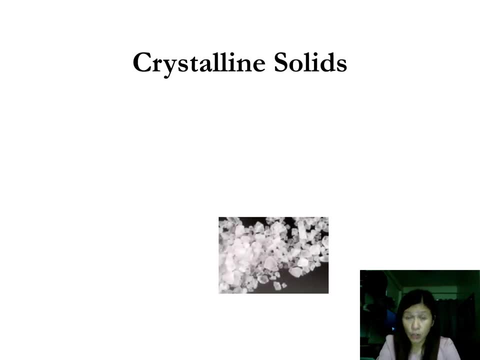 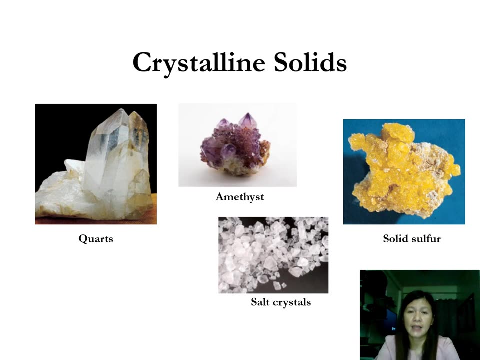 The Greek term amorphous is the origin of the word amorphous. This means shapeless, Going back to crystalline solids. these are the examples: We have salt, sulfur, quartz and amethyst. Amorphous solids are those that are in range order and whose particles occupy specific positions. 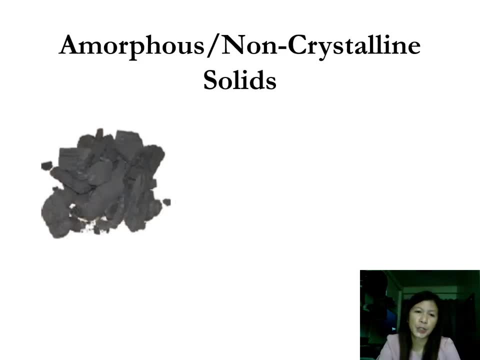 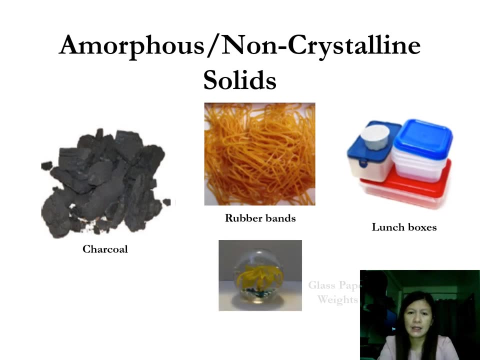 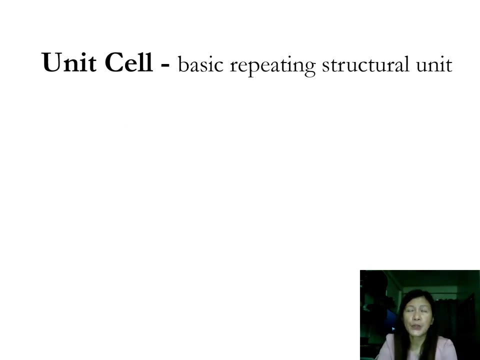 Now some more about crystalline solids. Amorphous are non-crystalline solids which may include charcoal rubber lording, some isoporous lambskin materials and ruby는데 rubber bands. lunch boxesised intentionally on paper and glass paper. 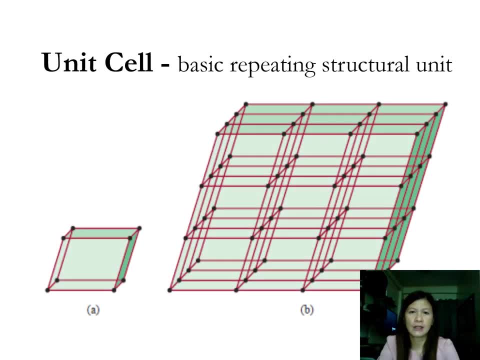 Looking back to the crystalline solids, these are characterized with unit cells. In letter A we have the smallest unit, the basic repeating structural unit of a crystalline solid, And in letter B, the repetition of the unit cell in three dimensions. 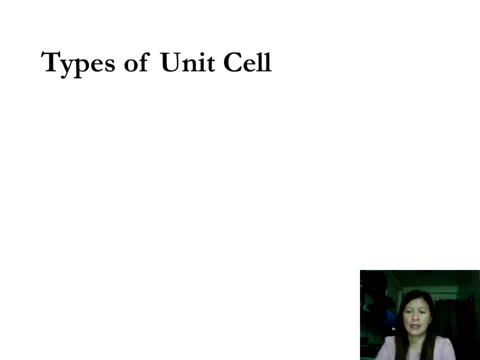 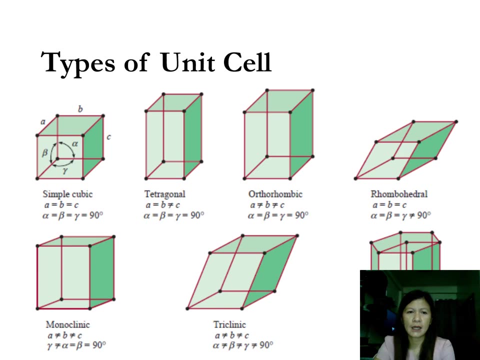 We have different types of unit cell. So you will see here the different types of unit cell, starting with the simple cubic cell. Notice the measures of the edges or sides, ABC, which are the same in simple cubic cell. We also have similar angles for alpha, beta and gamma at 90 degrees Celsius. 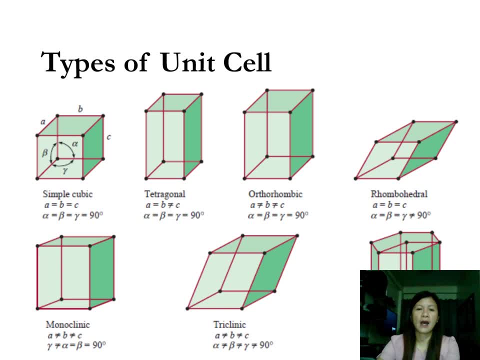 Another is tetrahedral, which have different measure of the C, different from edges A and B, But angles are the same, also at 90 degrees. Others include orthorhombic, rhombohedral, triclinic, monoclinic. 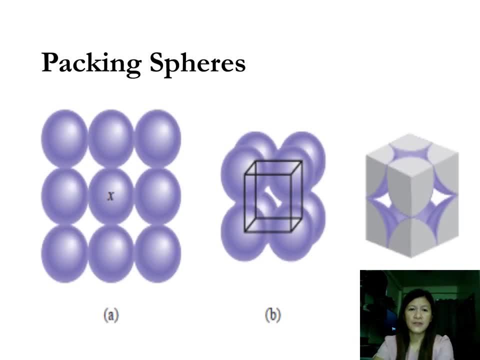 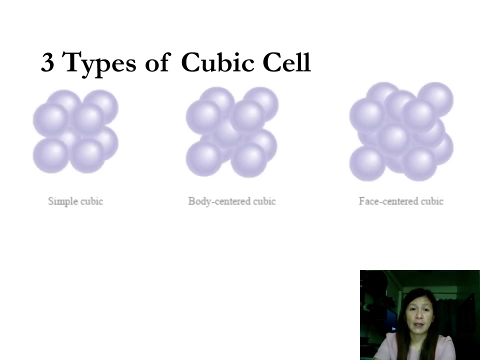 For the packing spheres. we have the illustrations here: A gives us the top view of the atoms in A simple cubic cell. B, we have the definition And C the cross section of each cell. We have three different types of cubic cells. 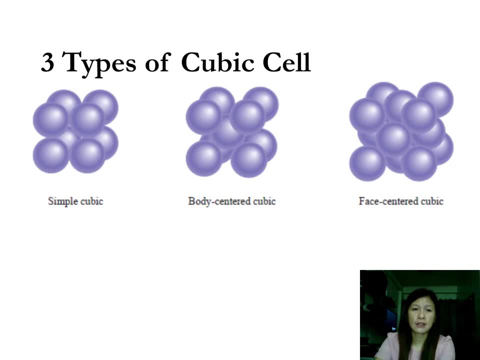 We have the simple cubic cell, or in short SCC, Body-centered cubic BCC And face-centered cubic FCC. Notice the number of atoms in each cubic cell. We have the smallest number of atoms or particles in simple cubic cell And the largest number of atoms in face-centered cubic cell. 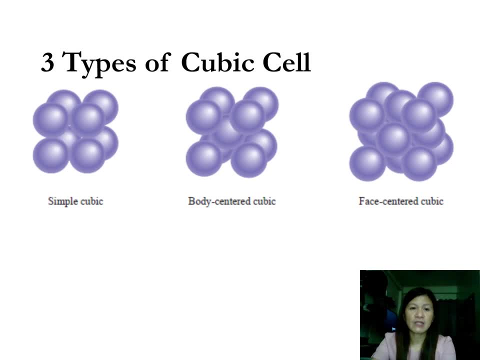 Notice that in each face of a simple cubic there are four atoms. In face-centered in each face there is additional middle atom, or atom in the middle, In face-centered in each face, there is additional atom. So in each face there are five atoms. 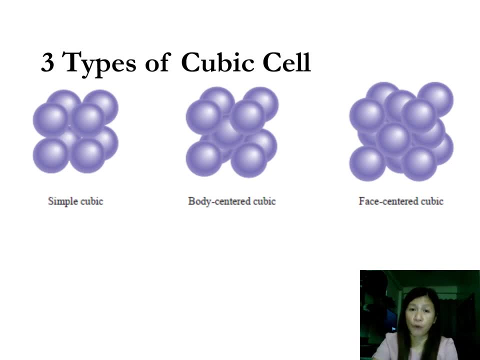 In body-centered there are four And one in the middle of all The. In simple cubic there is no central atom or atom in the middle of atoms in each face. So that gives the simple cubic the smallest number of atoms or particles. 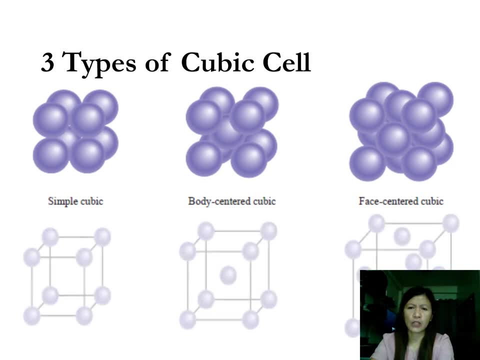 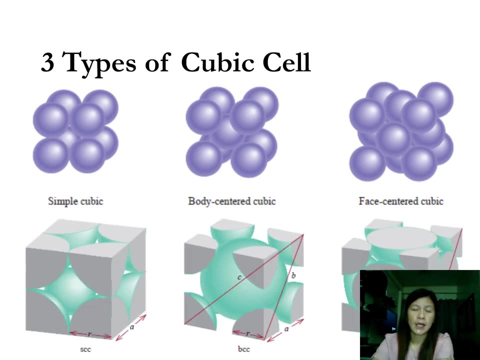 And face-centered, the highest number of atoms. These are the definitions of the atoms in each cubic cell And these are the cross sections. So notice the The number of atoms in the simple cubic cell. We have a total of eight atoms. 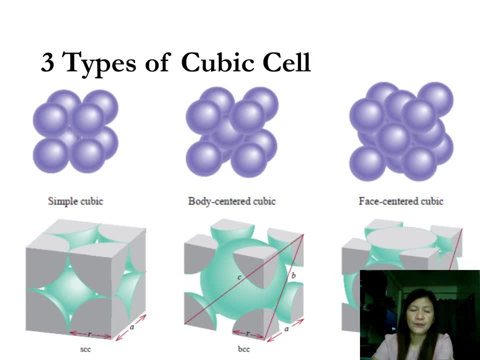 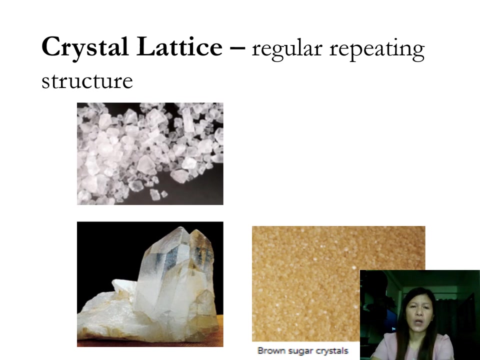 In BCC or body-centered, we have eight plus one, in the middle We have nine, And in body-centered we have six additional in the middle of each face. So that gives you a total of 14 atoms. And crystalline solids are also characterized with crystal lattice. 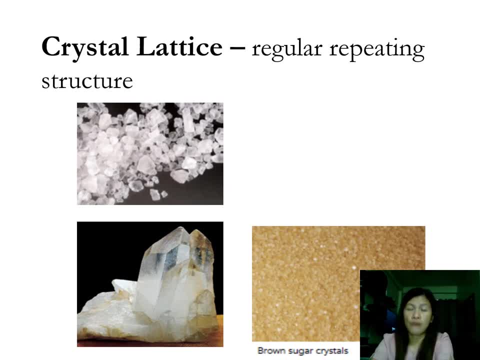 Crystal lattice is the regular repeating structure of crystalline solids. Again, these are some of the examples: Solid quartz. we have sugar. Other examples include ice- Ice as we are aware of when we look at it under a microscope. 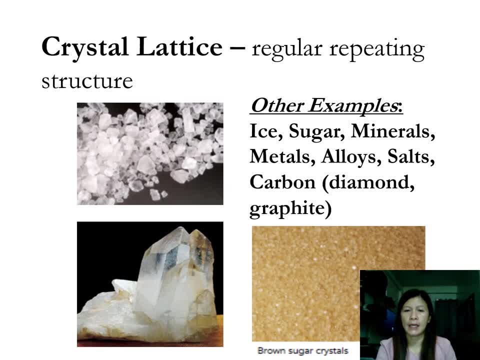 the ice has a well-patterned view of the atoms. So that's what happens when water is frozen: The atoms get a regular pattern. In fact, when it's Christmas, it's used as decor in malls or even in Christmas decor at home. 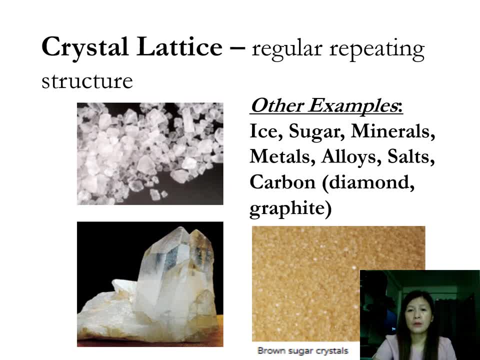 Okay, Sugar minerals, So the gems, the minerals that are mined. They are used for aesthetic purposes. So those are also examples of crystalline solids that are characterized with crystal lattice. We also have metals. Most metals, if not all, are crystalline. 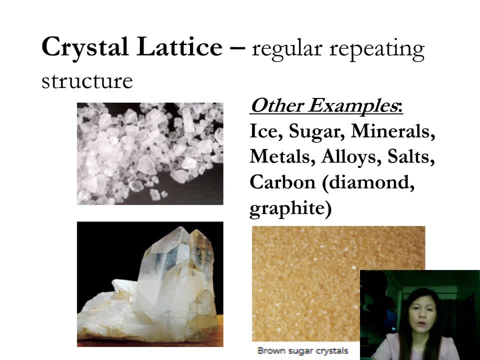 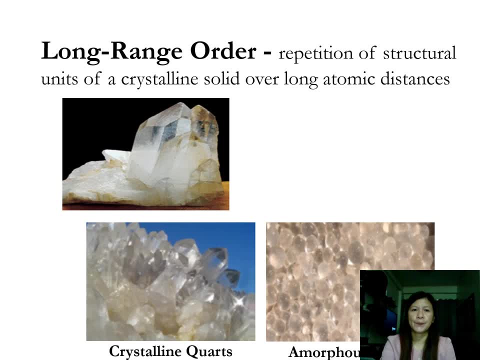 Alloys are mixtures of metals. We have salts, So sodium chloride is an example. Carbon in the form of graphite and diamond. Long range order is another characteristic of crystalline solids. This is the repetition of structural units of a crystalline solid over long atomic distances. 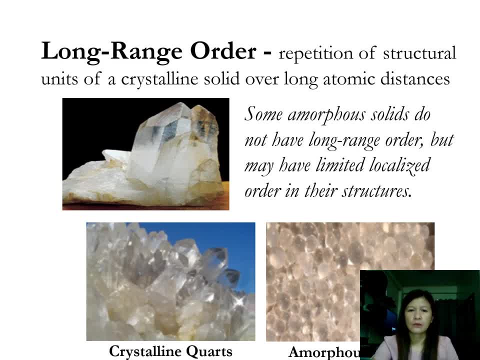 Notice here, quartz. Some amorphous solids do not have long range order but may have limited localized order in their structures, Like in the case of quartz. quartz have crystalline structure and amorphous structure. Speaking of amorphous structures, 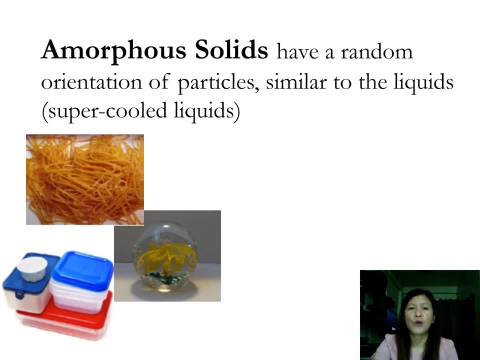 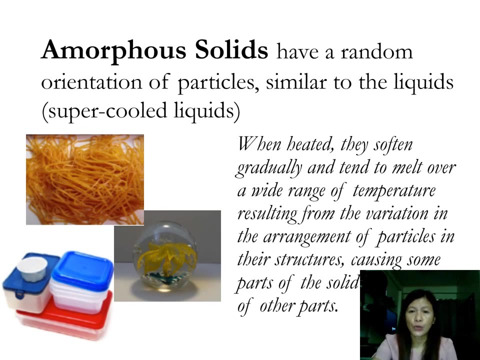 let's have amorphous structures which have random orientation of particles that is similar to the liquids and are sometimes referred to as super cooled liquids. Examples are rubber, glass and plastics. Take note also that when heated, they soften gradually and tend to melt over a wide range of temperature. 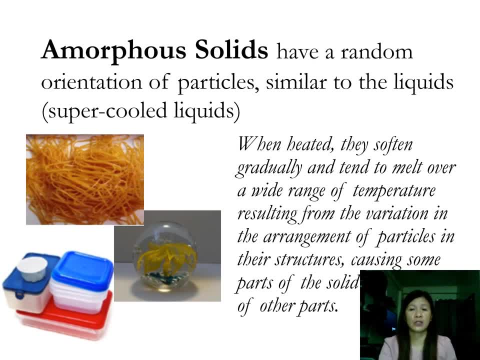 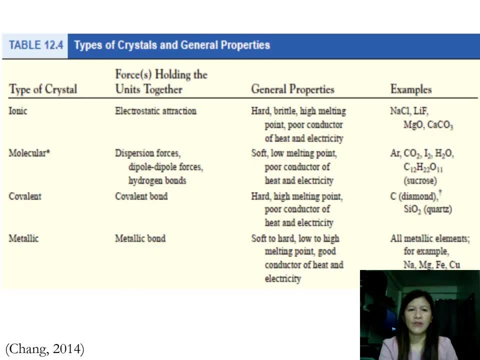 resulting from variation in the arrangement of particles in their structures. This causes some parts of the solid to melt ahead of time. These parts of the solid are the ones that will melt ahead of the other parts of the solid. You have different types of crystals, and the general properties are summarized here. 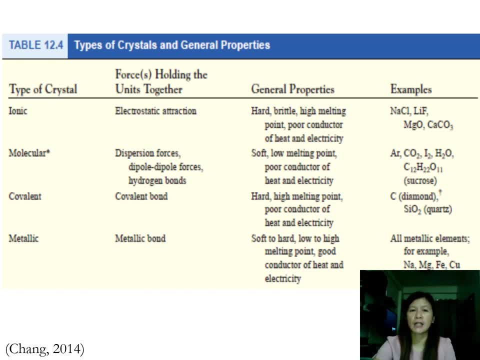 We have ionic crystals which are held strongly by electrostatic force. Electrostatic force is the force of attraction between charged particles. Examples of ionic crystals include sodium chloride, So most salts, lithium fluoride, magnesium oxide, calcium carbonate. General properties include the original sodium chloride. 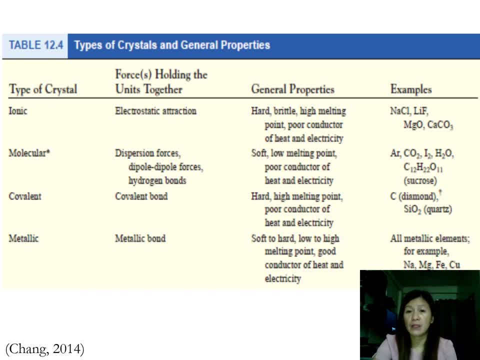 So most salts: lithium, fluoride, magnesium oxide, calcium carbonate. General properties include the original sodium chloride. They are hard, brittle with high melting points. because of strong intermolecular forces They are poor conductors of heat and electricity. Another group of crystals are the molecular crystals. 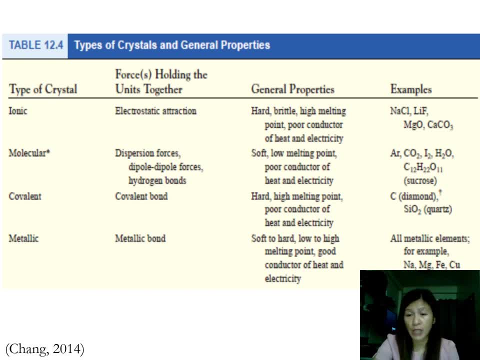 Examples are the solid argon, solid carbon dioxide, iodine crystals, solid ice and sugar. The strong forces holding them together are dispersion forces, dipole-dipole and hydrogen bonds. Their properties include: they are soft. they have low melting point because of weaker attraction when compared to ionic. 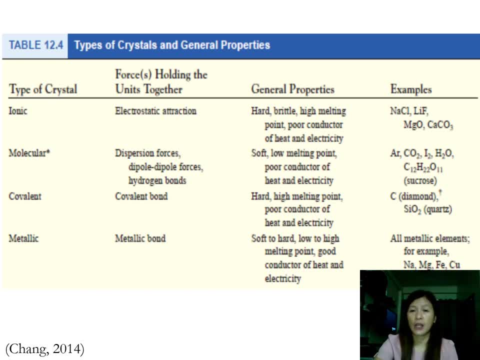 Ionic has strong electrostatic attraction. molecular have weaker IMF. That's why they have lower melting points than ionic crystals. Another type of crystal is the covalent. Covalent is a type of crystal that has a strong electrostatic attraction. 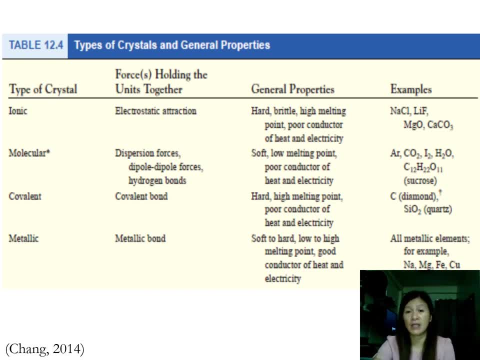 Another type of crystal is the covalent. Crystals are bonded, of course, by covalent bonds. Examples are diamonds and quartz. General properties: they are hard, So we know that the hardest mineral is diamond. They are hard. 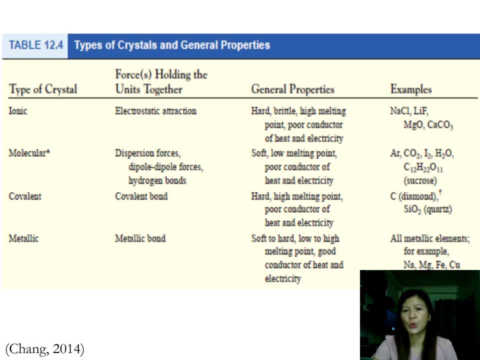 They have high melting points. High melting points is due to a rigid arrangement of particles. They are hard to break the IMF. They are poor conductors of heat and electricity. And the last type of crystal we have, the metallic crystal. Of course, they are strongly binded by metallic bonds, the strongest force of attraction. 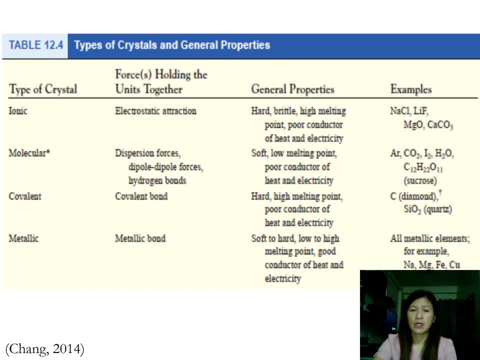 General properties include: they are ranging from soft to hard. We have metals that are soft like gold. They also have varying melting points: Low to high melting points. They are good conductors of heat and electricity. Among these types of crystals, metallic are the good conductors of heat and electricity. 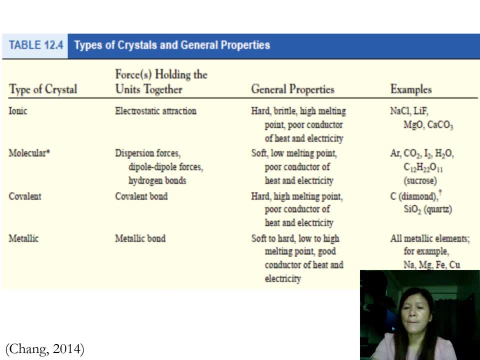 The rest are poor conductors. Also, they are generally hard compared to the other crystals, In exception, of course, with a diamond from the covalent group of crystals. In exception, of course, with a diamond from the covalent group of crystals. 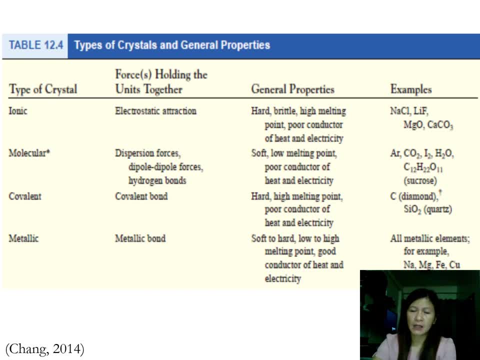 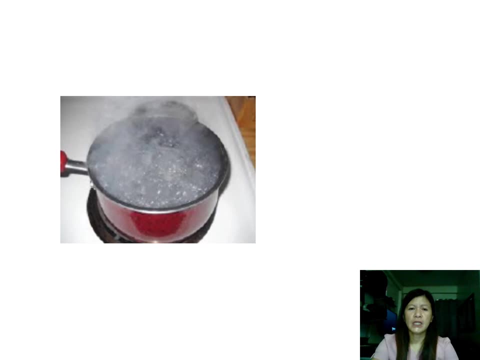 Some examples of metallic crystals include the metallic elements in the periodic table: magnesium, iron, copper, sodium and all the rest in your periodic table that are categorized as metallic elements. Moving on, what you see here is what? Yes, it's boiling water, melting ice. 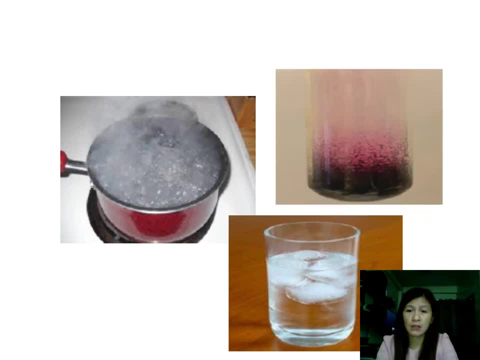 and the solid here that seems to be evaporating in layman's terms. and the solid here that seems to be evaporating in layman's terms, But actually scientifically it is more appropriately described as subliming. So solid, subliming or turning into gas. 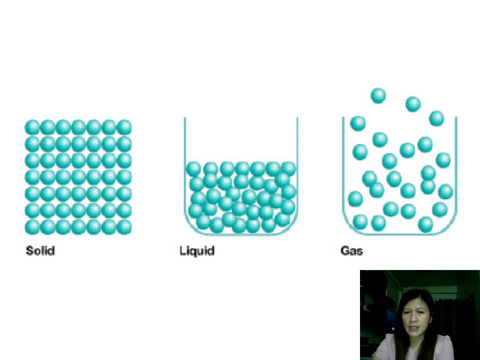 To recall the arrangement of particles in solid-liquidine gases. of course we know that solid particles are closely packed. Liquid particles are having spaces between particles. Liquid particles are having spaces between particles- They are not in close arrangement And gases are in the widest separation. 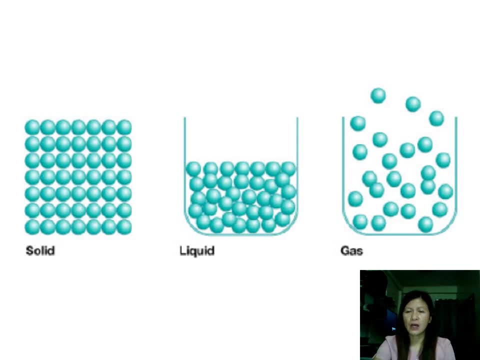 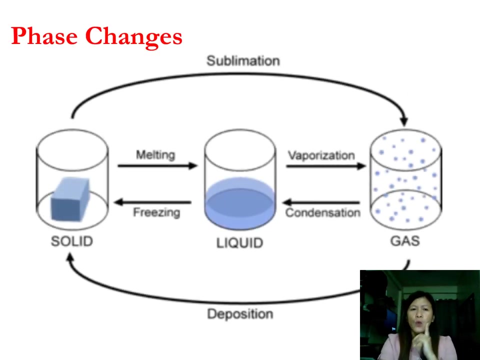 the widest separation. so among the three, the strongest attraction is in solid, because they are well packed, and weaker attraction in between gas particles. when does water or liquid turns to another phase? or generally, when does sample of matter turn or transform from one place to another? so we have what we call the phase changes. so you will see in this diagram the summary of the 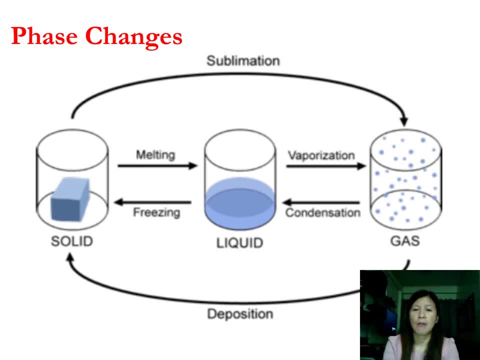 transformations, the different transformations in matter. so again, we have three states of matter generally. we have solid, liquid and gas. we have six, a total of six, phase changes. we have two reverse processes, another two reverse processes and another two reverse processes. let's start with the solid matter. 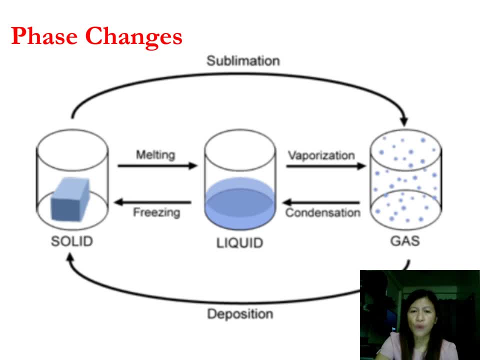 or solid state of matter. when solid transforms to liquid, the process is known as the phase change, is known as melting. the reverse process of melting, that's, transforming liquid to solid, is called freezing liquid. turning to gas: we have vaporization, gas turning going back. turning back to liquid is condensation, but it is a solid solid transforming to 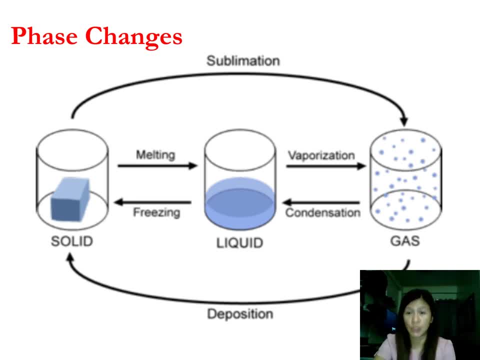 to gas without passing the liquid state is called sublimation, and under certain conditions gaseous matter may transform to solid, also without passing the liquid state. so we have the reverse processes: melting, freezing, another vaporization, and condensation and sublimation and deposition. the question is, when does a state of matter or matter changes? 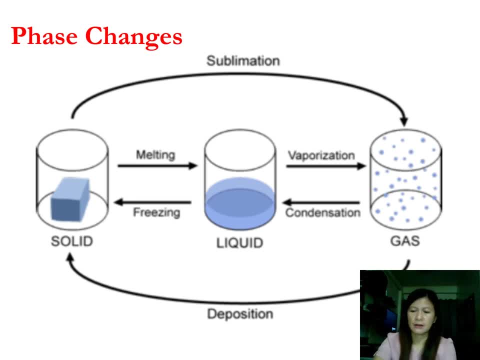 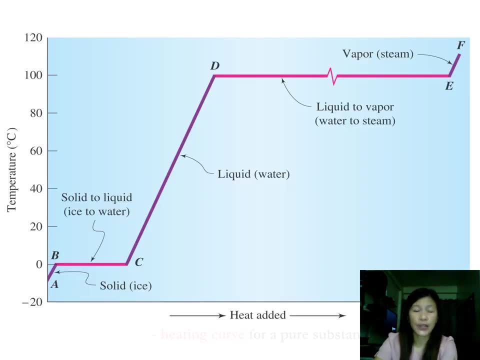 change from one state to another. you are correct. temperature, temperature phase changes. we have here the heating curve for a pure substance. so what you see here are the temperatures along the y-axis and um heat added along the um x-axis. so what happens? let's take water as an example. commonly used example is water to to illustrate the 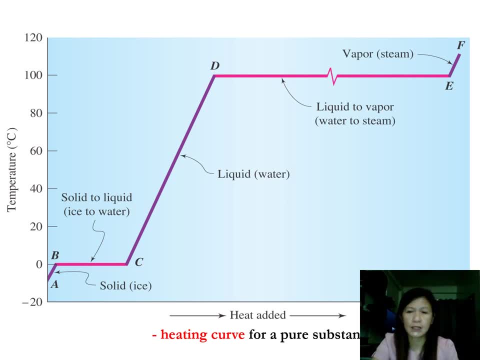 uh, the transformation of matter from one state to another. below zero degrees celsius. water is in the solid state in the form of um ice. so solid water, called ice, is under zero or below zero degree Celsius. when does water? or solid uh water in the form of ice? 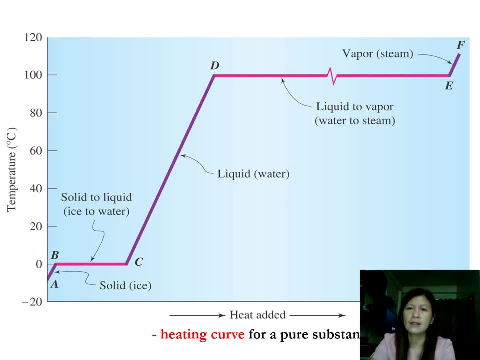 uh, when will all of this formalize ice melt, or when can it melt? first, ice needs to absorb heat energy. that amount of heat energy needed to increase its temperature from negative degrees Celsius to zero is what we call the Latin heat of fusion. so that amount of heat is necessary to increase the temperature from negative to zero. 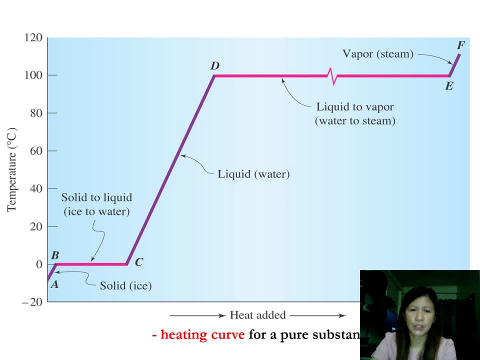 degrees Celsius, and then at zero degrees Celsius, ice will start to melt. so notice here, from point A to B there's heat absorption. so from a possible detour, Latin heat of fusion, the amount of heat necessary for the sample matter, in this case ice, to absorb in order to increase its temperature from. 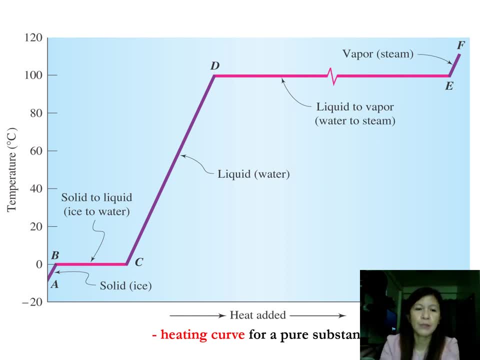 certain negative degrees Celsius to zero. hindi po siya aakyat to zero degrees Celsius unless mag absorb ng heat energy yung ice. at that point, at point B, where the temperature is already at zero, ice is expected to start melting. notice the points B and C. solid water or ice is turning to liquid at that point or at these. 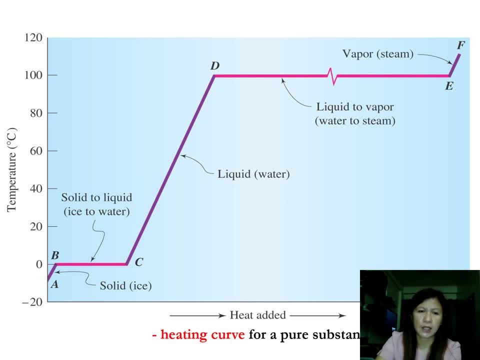 points notice: temperature is not changing. it remains at zero degrees Celsius. take note that during the course of melting or any phase transformation, temperature remains at. let's say, in the case of ice, it will remain at zero. Kailan po hihinto na or kailan siya aakyat ng temperature Once ice has completely. 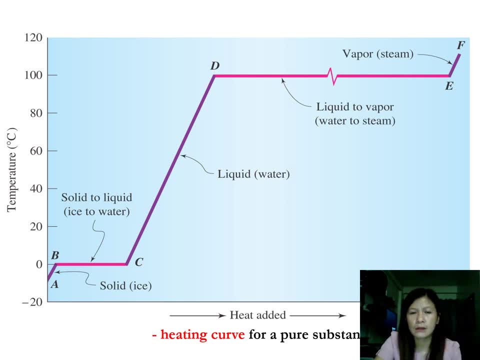 melted, saka lang siya mag-start magbago ng temperature At para magbago yung temperature niya para tumaas kailangan ulit niyang mag-absorb ng heat energy. So notice the change in heat absorption across the x-axis. So meron kang increase of heat energy from point C to point D. 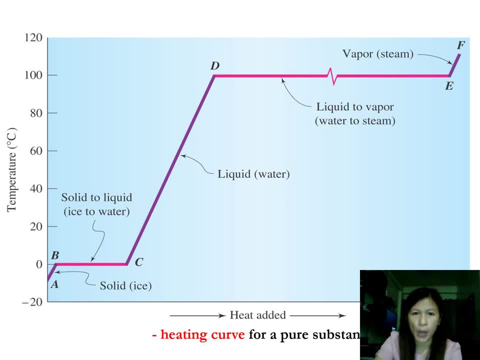 There's absorption At these points. nagkakaroon ka rin ng increase in temperature. So you started from point C, that's zero degrees Celsius, As heat is being absorbed by a melted water or melted ice that is already in water. nagkakaroon ka ng rise. 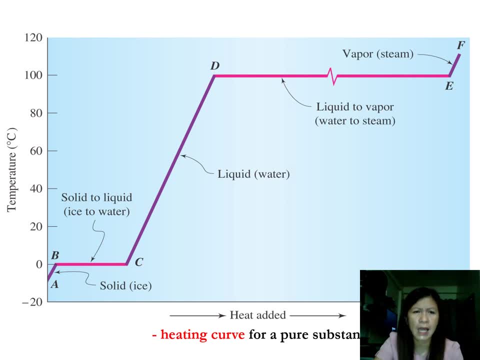 In temperature to 20,, 40,, 60,, 80, until you reach 100 degrees Celsius, And at this point your water will stop changing its temperature Kasi mag-start na ulit siyang mag-transform into another phase. So that's what I meant when I mentioned about temperature remaining during the 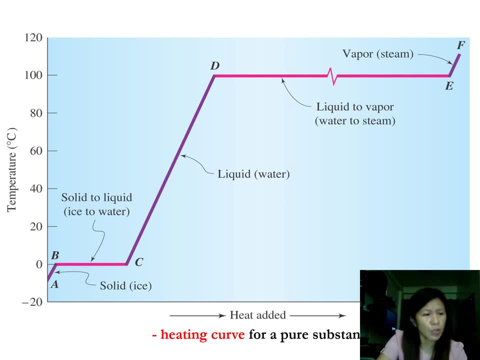 course of phase transformation. So pag natutunaw siya, pag nagbe-melt siya, hindi siya nagbabago ng temperature. Pag natunaw na siya, sakalang aakit yung temperature niya until such time that it will start transforming naman from liquid to gas, And at that point 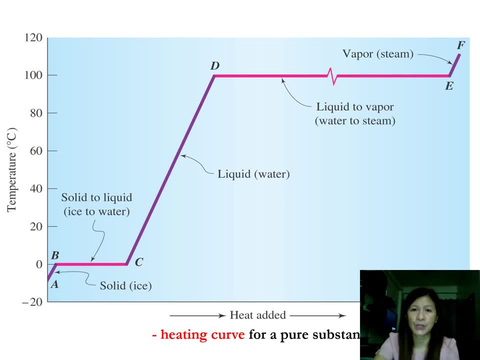 during evaporation. hindi na ulit aakit yung temperature niya, mananatili na ulit siya sa 100 degree Celsius. And that will continue until all the water molecules have transformed into gaseous form or gaseous state. So after: 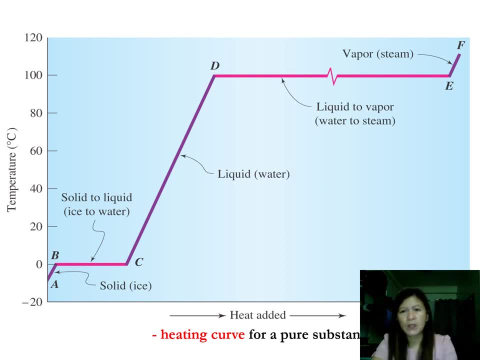 mag transform na completely from liquid to gas, umpisa na ulit aakit yung temperature nya and it will start again to increase its uh heat energy absorption. so, as you can see in the um heating curve, so from point e, from point from point d to e, there's constant temperature. 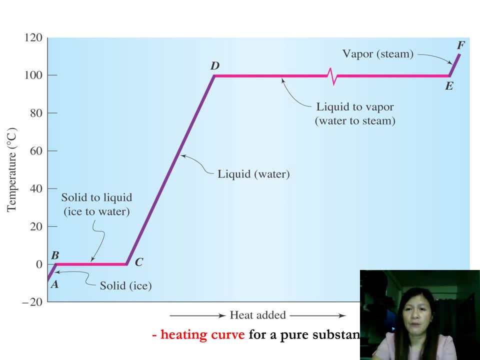 400, because that's the course of evaporation, pero from e to f, that's um transforming or absorb a vapor, water vapor continuing to absorb heat energy, changing its temperature from 100 to a higher temperature. so that's what how we interpret the heating curve for a pure substance. 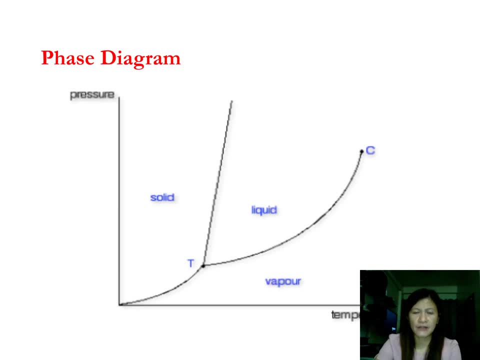 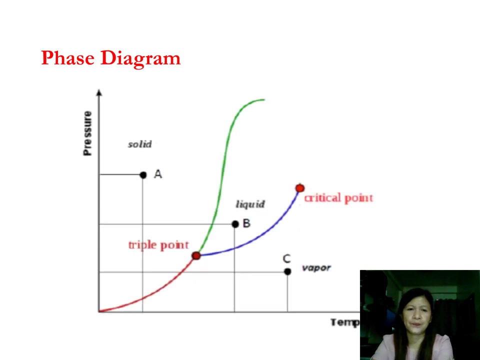 another graph is called the phase diagram. the phase diagram shows the states of matter and the critical point and the triple point. critical point and the triple point are two important concepts that we need to take note of when considering the transformation of matter from one phase to another. okay, along the y-axis, you see the 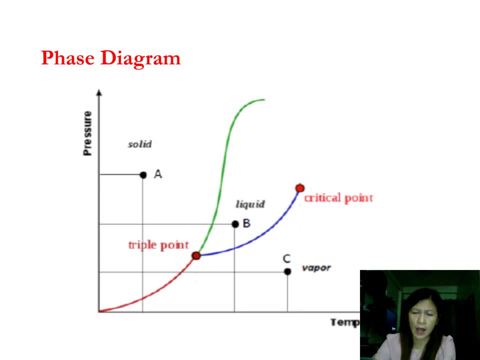 you see pressure along the x-axis. you have the temperature. so it's a pressure temperature graph or a simply phase diagram. so you see the three states of matter. here we have the solid liquid and gas. tapas mero can become lines the door and you know we have red, blue and green. so yung yung uh. boundaries is important here in this case the azจung yi. then we see almost all or NO water في diール. they contain three different forms of gas that have three different colors. what you use it for will be according to the legacy and type D of the point there, so it will be according to sexual elaborate on this graph. that will split the level of temperature chances that you must choose different areas of freshness or 됩니다. natural abstinence or some of the forms will be relevant. it may have a minimum tolerance. there will be changes or very small differences of water quality and technical properties of water and temperature. If there are plenty of primary places on your water content, there's also a limit on that. 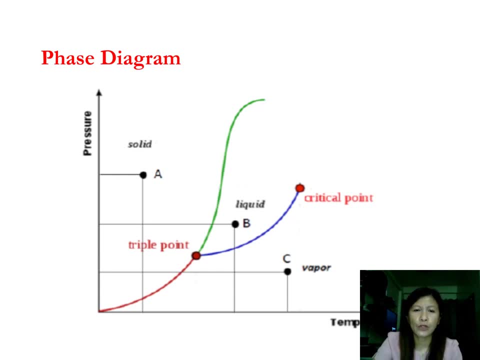 nila. so from the zero mark to the triple point is the continuous increase in pressure and temperature. that triple point is the temperature and pressure at which a certain uh substance co-exist as solid, liquid and gas. so that's the temp, that's the point. for where in the temperature? 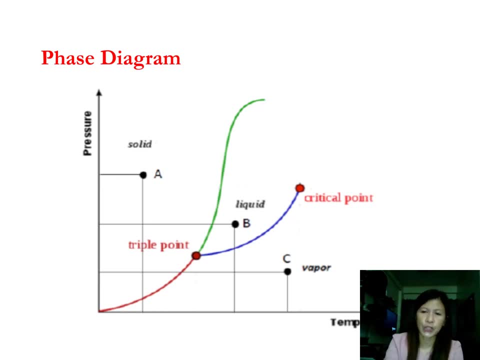 and pressure, wherein at that temperature and pressure yung three states of that sample of matter co-exist. so we call that the triple point, critical point. so in between, so it don't line up. it don't line up from the triple point at yung green na yun, ayun naman po yung boundary, or 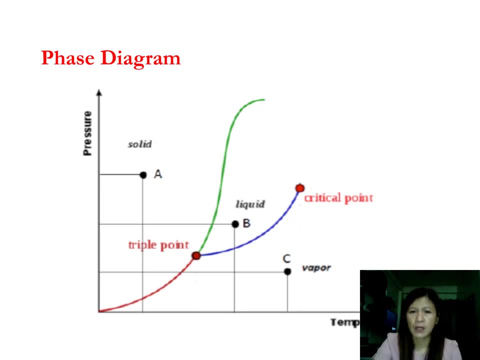 demarcation between the solid and the liquid state, from the liquid state to the to the gaseous state. ang boundary naman po nila ay yung blue. the critical point terminates the transformation of um liquid to gas. that's the highest possible temperature that the liquid can. 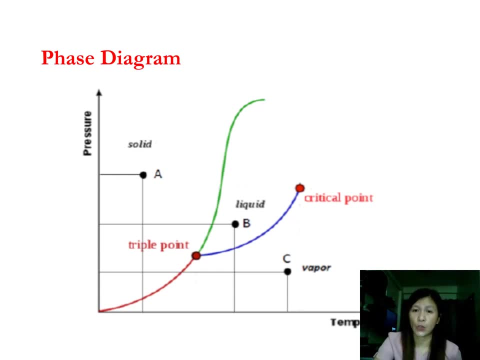 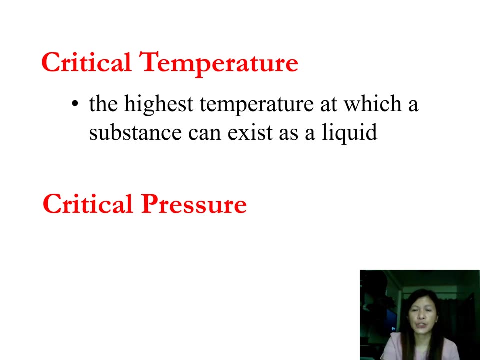 can can exist as liquid. so we call that the trip, the critical. so again, critical temperature is the highest temperature at which a certain substance can exist as a liquid, because beyond that hindi na siya pwede mag exist as liquid, mag magta transform na siya whether it likes. 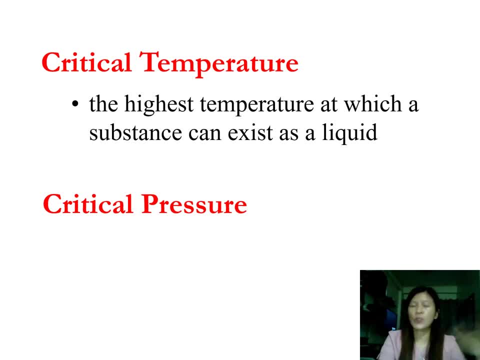 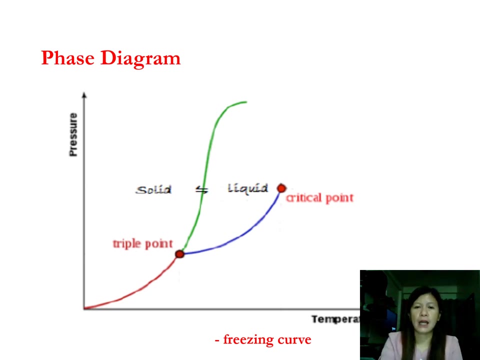 it or not, to gaseous state, so it will continue to. to transform to gaseous state critical temperatures, that is the minimum temperature pressure that uh must be applied to bring about liquefaction in the critical temperature. kaya lagi po silang partner? okay, let's see here the freezing curve. 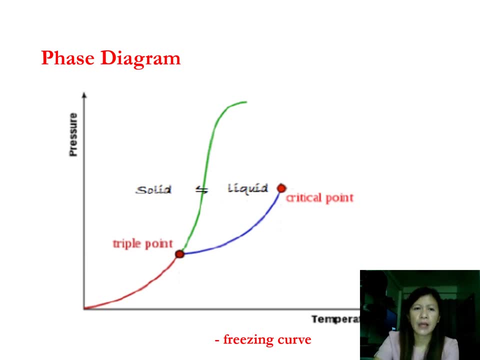 freezing curve of a substance. take note, by the way, that each substance has its own phase diagram, so distinct po ang mga phase diagram ng mga substances. for example, water has its own phase diagram, carbon dioxide has its own phase diagram, sugar has its own phase diagram, and so on. 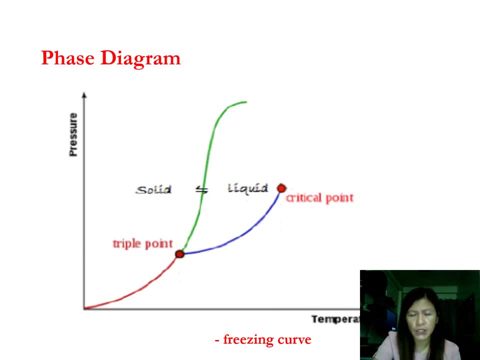 and so forth. so for this particular example, generally, uh, general example, freezing curve. so we see here: solid transforming to liquid. anywhere in the green line, equilibrium po exists between melting and freezing. so between these two reverse processes- solid to liquid, liquid to gas or melting and freezing, anywhere in the green line, equilibrium exists between melting and freezing. 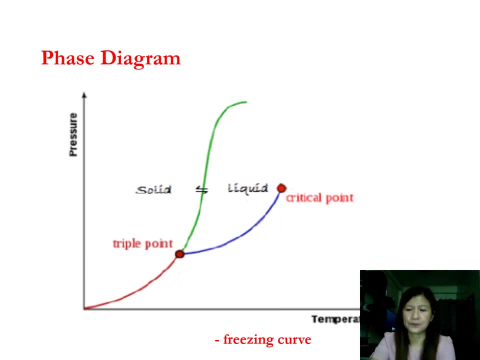 between the two phase changes, on the other hand, between another two reverse processes: evaporation and condensation, that's, liquid to vapor and vapor to liquid in anywhere in the line blue line exists equilibrium between vaporization and condensation. what do i mean with equilibrium? magsing bilis po yung. 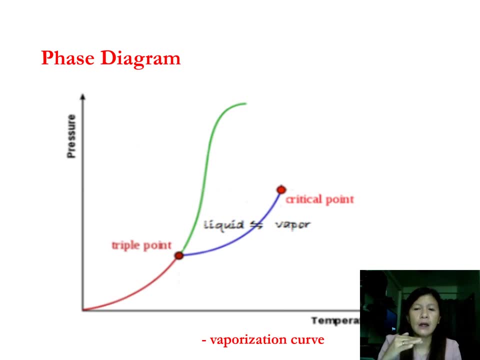 proseso yung, yung, yung bilis ng evaporation and condensation. so that's what we mean by equilibrium: both evaporation and condensation- or, in the previous slide, freezing and melting- exist at same rates. at same rates, i'll repeat: the critical point is the point that terminates the 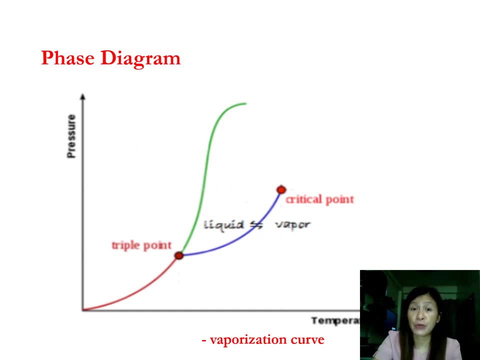 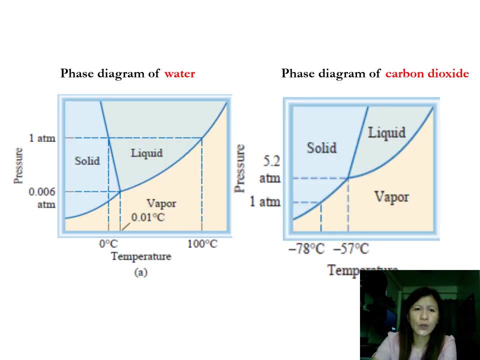 um. evaporation or vaporization or transformation of liquid to vapor. termin determinates the: the transformation of liquid to vapor of a certain by a certain liquid or substance. let's take a look at the phase diagram of water and carbon dioxide. let's have water. we all know that the freezing point of water is similar to its melting point, which is zero same. 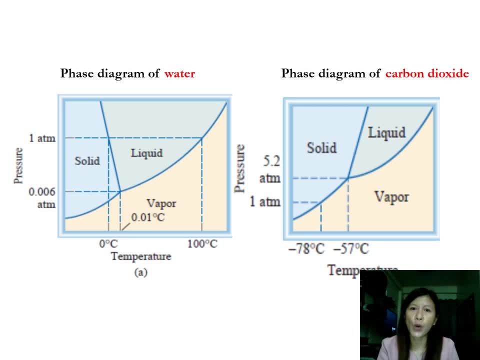 with um evaporation, boiling point at 100 degrees celsius and a condensation point at same temperature. so freezing and melting temperature it remains at zero degrees celsius, same with vaporization, while na transform ang liquid to gas hindi rin nagbabago yung temperature, Basta during the 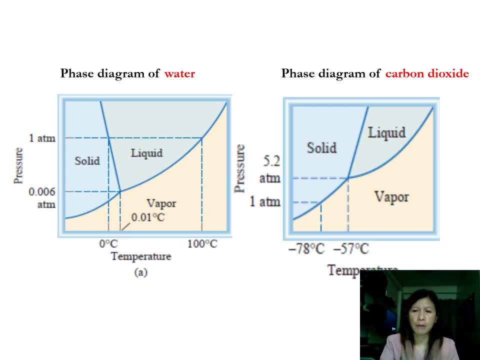 course of phase transformation, temperature remains the same. Okay, Hanggang sa maubos na yung substance from one phase nag-transform na completely to another phase. Saka lang siya mag-i-increase ulit ng temperature until such time na kailangan niya ulit mag-transform. 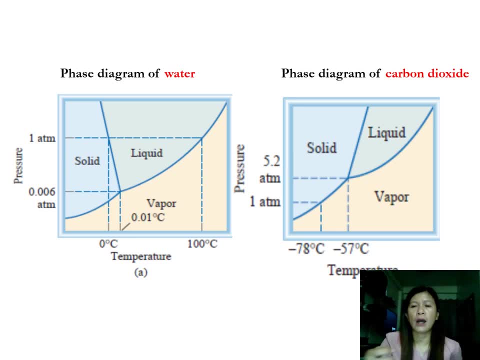 into another state of matter. Same with removal of heat. Hindi lang naman yung pagtaas ng, pwede rin yung pagbaba ng temperature to transform, let's say gas to liquid or liquid to solid. So same thing lang. Hindi lang palaging absorption ng heat. 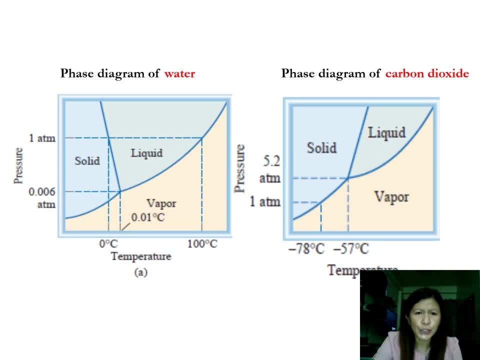 ang senaryo. Okay, So notice here: at normal conditions, 1 atm and 0 degrees Celsius, water is at sorry sorry. at 1 atm and 0 degrees Celsius, water is in the solid phase or in the solid state. At 100 degrees. 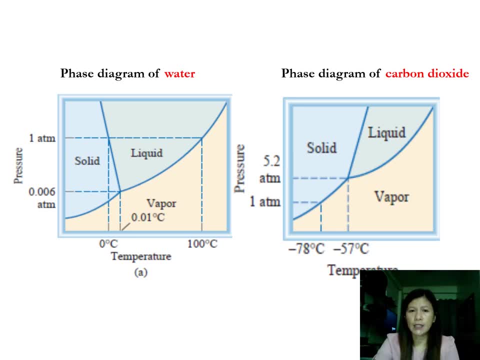 Celsius and 1 atm water is at liquid phase. Okay. Pero in these normal conditions, 1 atm the physical state of carbon dioxide. let's have. 1 atm, it's solid, Okay. So in this example, carbon dioxide is solid at zero degrees Celsius, 1 atm at a very low temperature of. 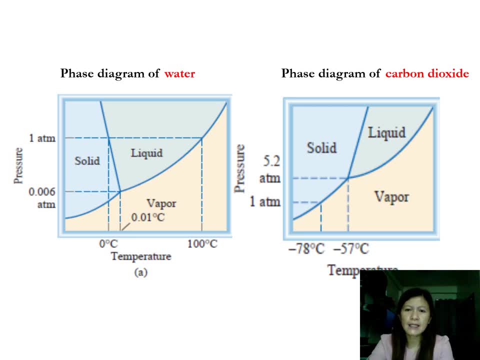 temperature of negative 78.. Let's have the liquid state At 1 atm. sorry, at 1 atm and at it can never be possible that carbon dioxide will exist as liquid at same conditions as water that exists in liquid, If water exists as liquid from 1 degree Celsius, for example. 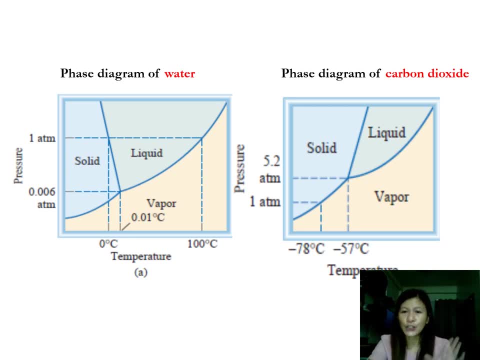 ang carbon dioxide ay hindi. It has to reach what Higher than negative 57 degree Celsius? negative 57 degree Celsius and at a higher, at a much higher pressure. Kung ang water requires only 1 atm and about 0 degree Celsius to become liquid, ang carbon dioxide ay hindi. It requires higher pressure. 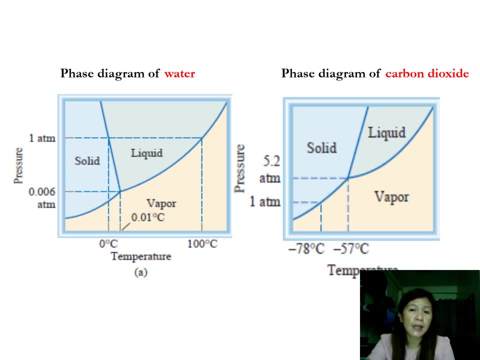 5.2 and at least 56, negative 56 degree Celsius para mag-exist siya as liquid. So under normal condition, carbon dioxide is indeed solid and cannot come in a liquid state, So it can't be liquid. That's why carbon dioxide is referred to as dry ice. That's the reason. Look at the critical.